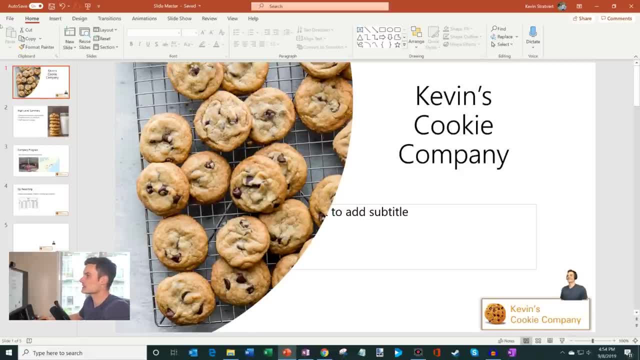 as a video. So how do I go about doing that? So the first thing that we're going to do is click on this pivot option that says slideshow. So I'm going to go ahead and click on that And then under here you'll see an option right under the slideshow pivot that says record. 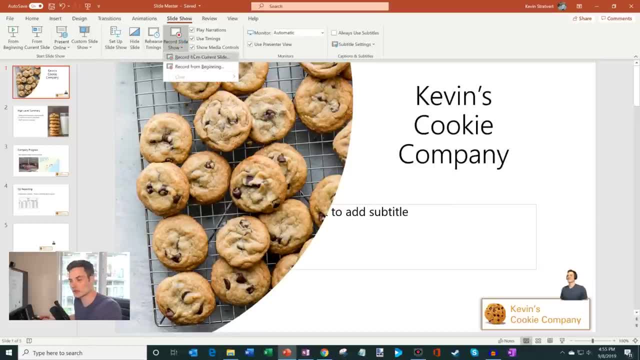 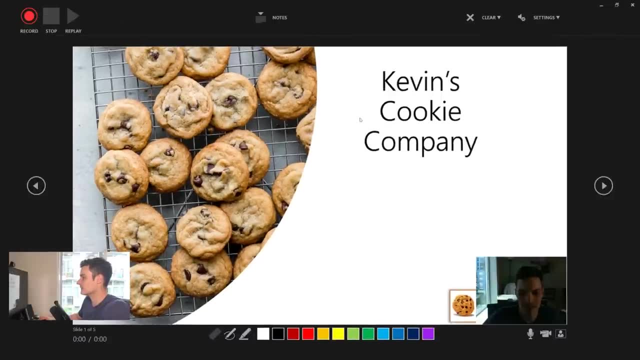 slideshow, And what I'm going to do is you could either record from the current slide or from the beginning, but in this case the current slide is the beginning, So it doesn't matter which one I choose, So I'm going to go ahead and say from the beginning. Now a few things that I could do on. 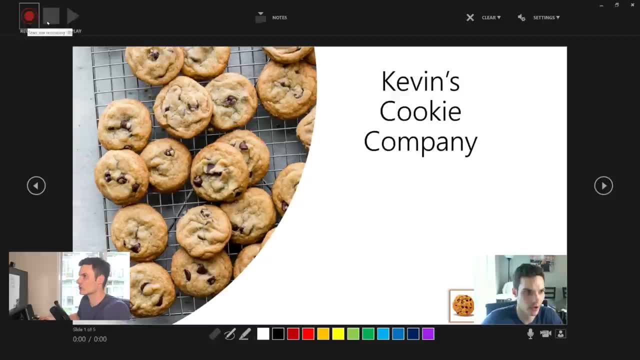 the screen that popped up, you see this big red record button. Well, that's how I record. I could also stop recording and then I could also play it to hear how it sounds. I have some settings under here where I could choose my microphone. I could choose my camera. 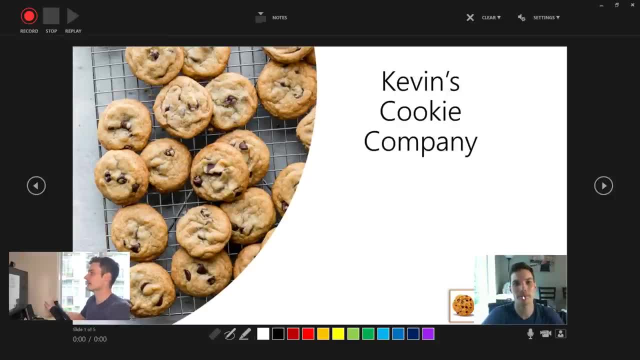 In this case, you see me showing up on here because I'm using my webcam to get my video onto this slide, And you have options where you could turn your microphone on and off, your camera on and off, and you could turn on the preview or not the preview. So it's kind of cool because what I 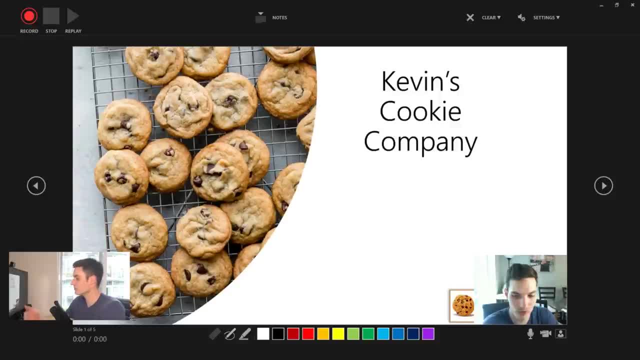 could do is I can record myself going through this presentation, speaking through it, and people could also see me on the video, So it's a really nice format for, say, a YouTube video. What I can also do as I'm going through it is I also have a pen and I have a highlighter, So here I could 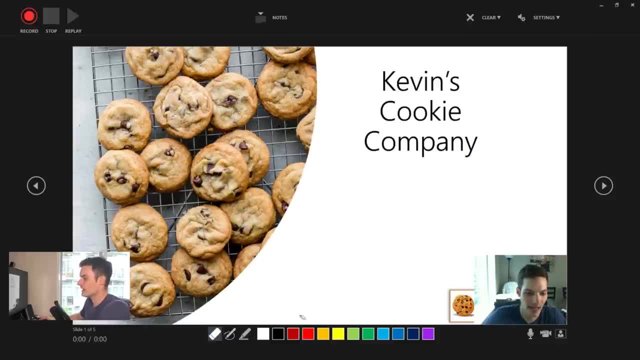 highlight my video and I can also record myself going through this presentation. So here I can highlight things on my slide as I'm going through it And those different animations will show up as I go through the slide. So let's give this a shot, And I could also show notes if I want to. 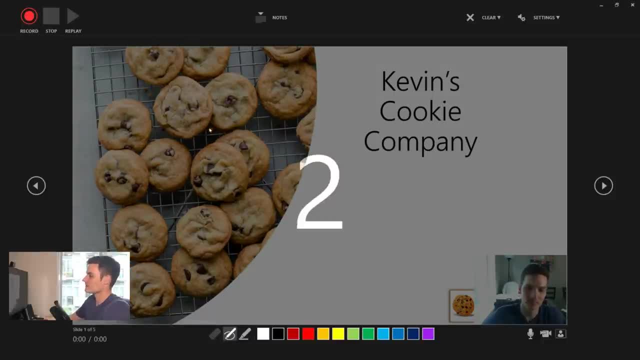 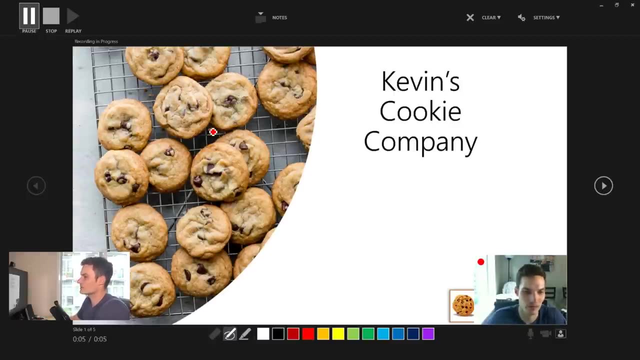 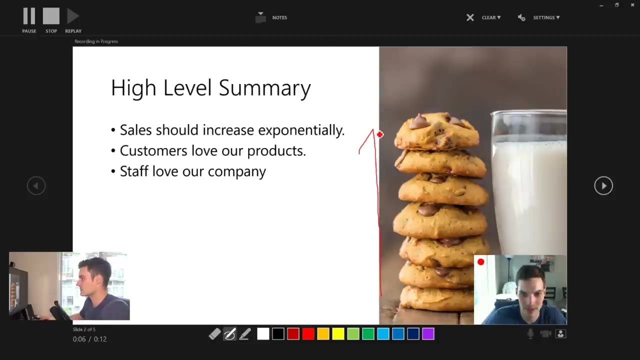 Okay, so let's go ahead and record. Hi everyone, My name is Kevin with Kevin's Cookie Company, And today I wanted to walk through some of our recent results that we've had with the cookie company. Now sales have really been growing exponentially. You see, these cookies. That represents our growth right there. 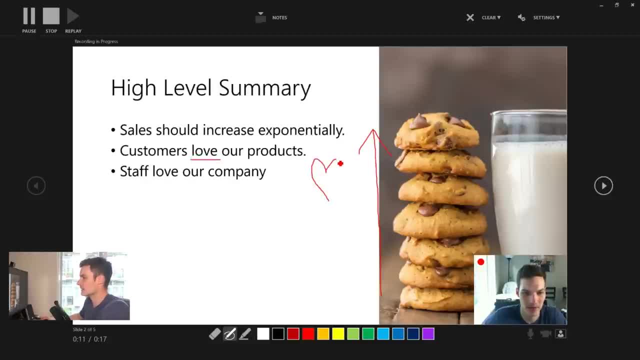 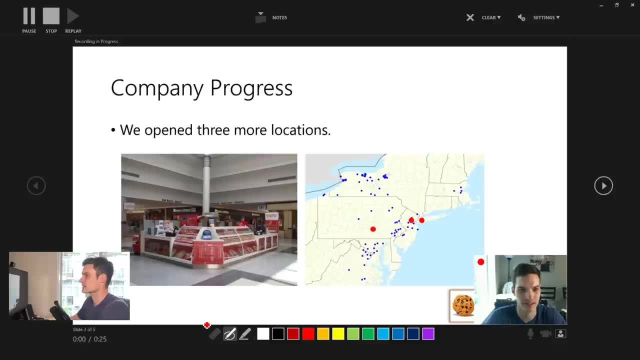 And really customers love our products. When I say love, I mean they really love these cookies. And also, not only do our customers love our cookies, but our staff love working for this company. In fact, people love us so much that we've been able to open three additional locations. 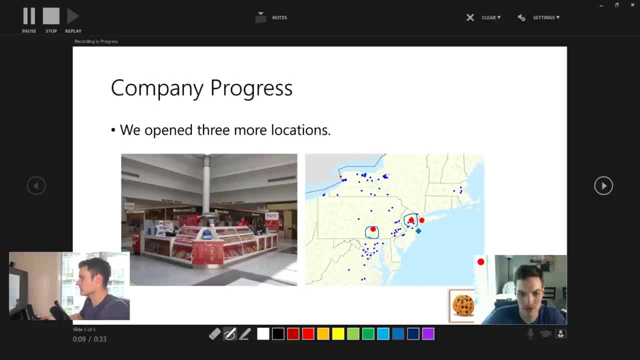 We have a location that we recently opened up in Pennsylvania, We have a New Jersey location And we have a New York location, In addition to all these other blue dots. we are a very big company, because look at all these locations all over the. 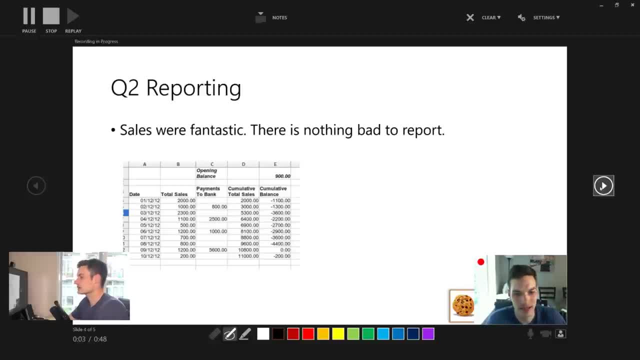 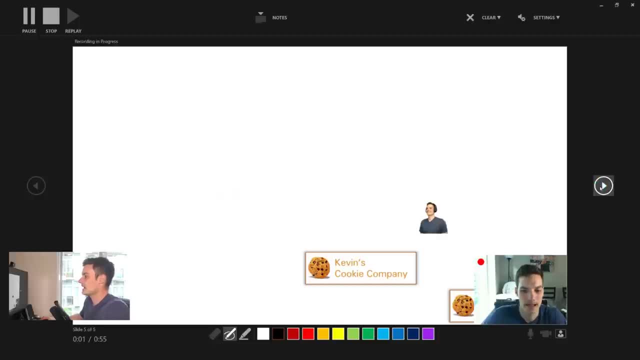 app. Now, when we look at sales, sales have been doing fantastic. There's really nothing bad to report. We've had just amazing performance. And that wraps up the presentation. So, now that I've finished the presentation, what I'm going to do is I'm going to click. 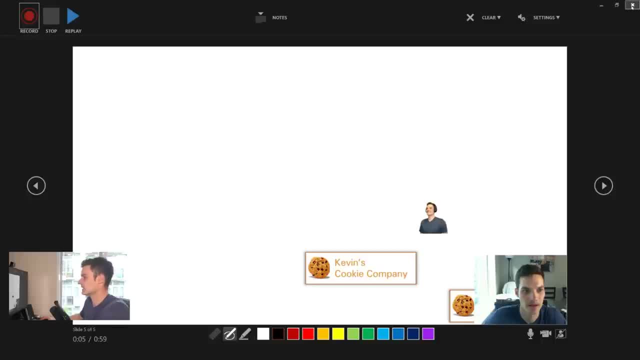 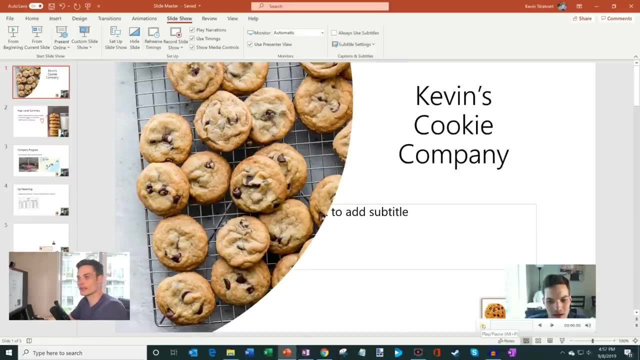 on the stop button and now what I can do is I can just close this out And you can see the total recording was about one minute long, so I'm going to hit this X button. Now that I've finished recording it here, I am back on the main slide view and on each 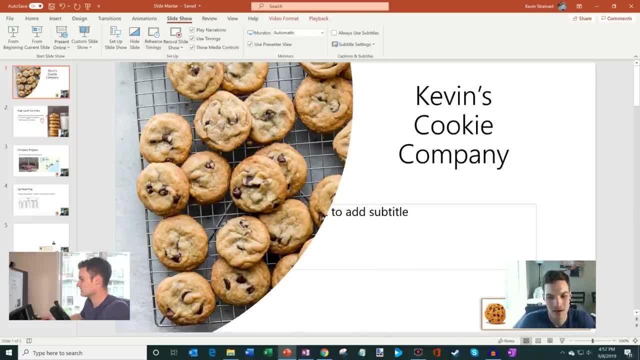 slide. now you see a video that I can move around to different locations. This is my video of me talking, and each slide has that, And what I could do is I could simply click on this play button. And so now what I could do is I could send the deck out to someone and they could go. 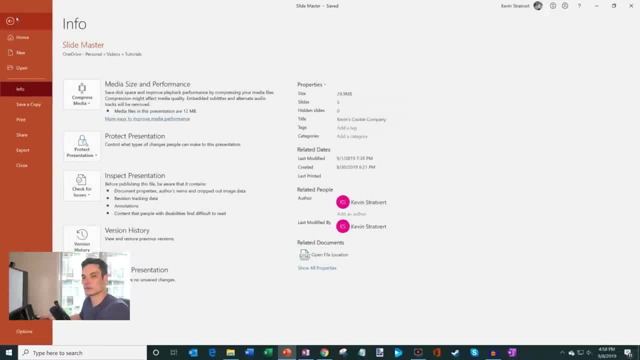 slide by slide and they could see my recording. Or what I could do is, if I want to prep it, where it's just kind of a package that I could send off to YouTube or Facebook or Vimeo or wherever I want to share this now I could. 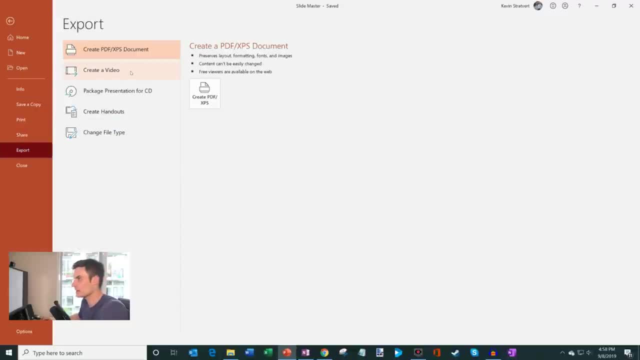 simply click on export And create a video. So what I'm going to do: create a video. You could do it in Ultra HD, which is 4K or 1080p. So I'll just do 4K and I'm going to create the video. 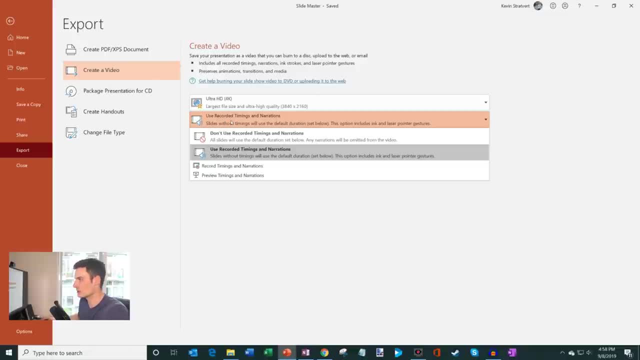 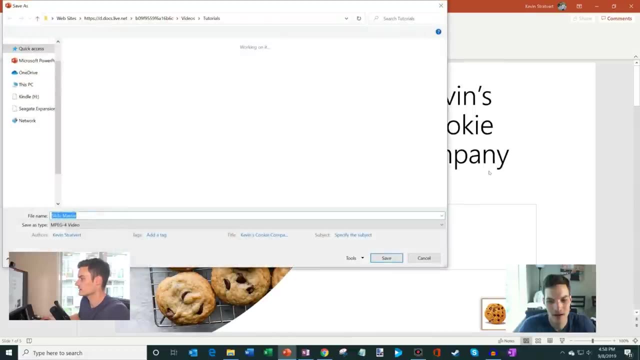 And what it's going to do is I'm going to use my recorded timings as I was going through it, and I also want to use my narrations. So sure, sounds good, Let's create the video, And now I just have to choose a location. 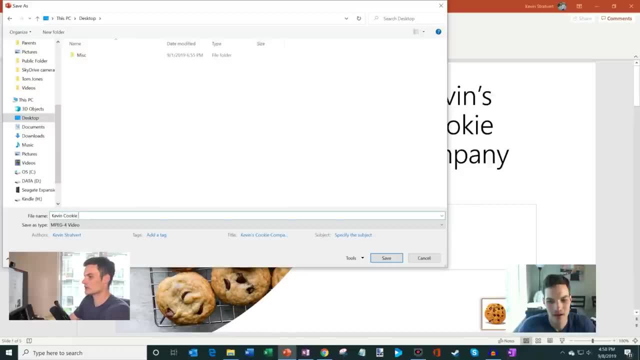 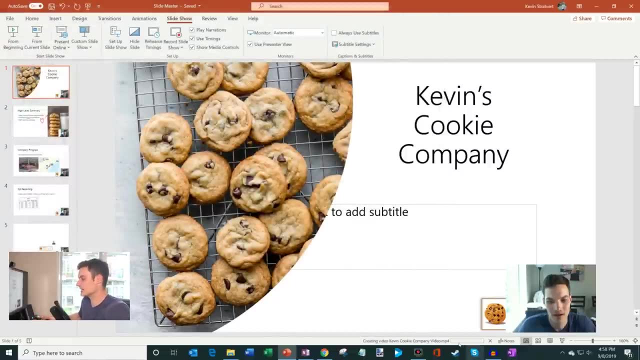 So I'm going to put it on my desktop and we'll say we'll just call this Kevin Cookie Company Video And let's put it on my desktop. It's going to take a little bit of time to go through. You can see in the bottom right hand corner. it's rendering the video and, depending on 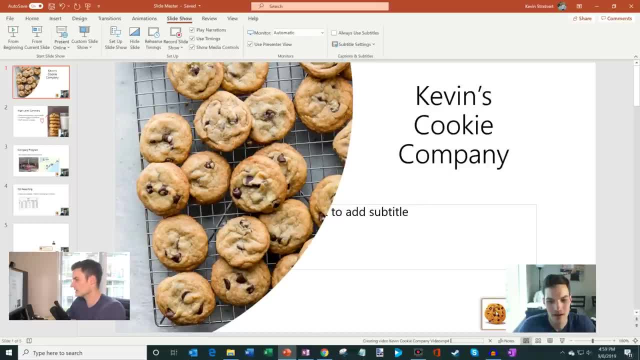 how long it is, how many slides you have, how much video narrations included. it might take a little bit longer to go through and render, so we'll just hang out for a moment until it's done. How long is this video render going to take? 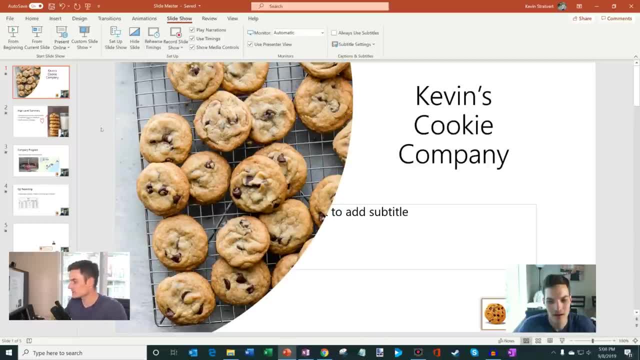 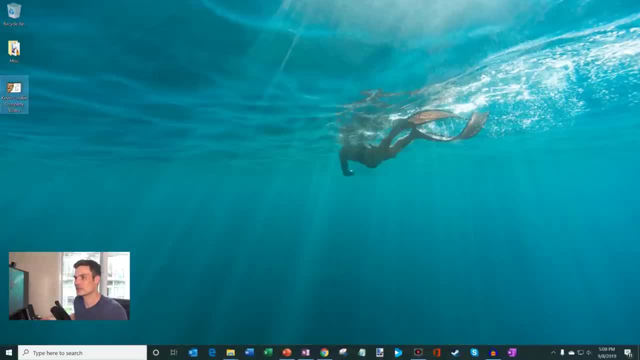 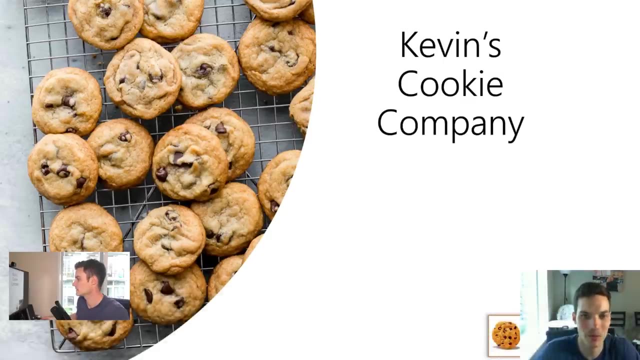 I don't know. It's going kind of slow. Looks like it has finished rendering the video, so I'm going to go ahead and minimize PowerPoint And go back to my desktop. I saved the video file to the desktop and let's play this.